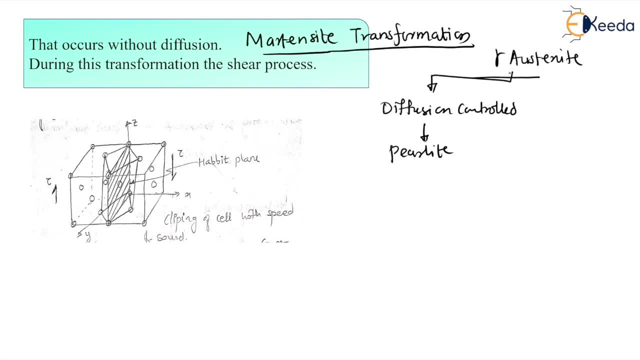 And, dear students, when we have the diffusion, less transformation, very important, diffusion, Diffusion, less transformation. So that time we will be having the martensite, martensite phase. okay, And, dear students, if I put here the interrogative sign- okay, that is, I am serious, there will be the bainite, there will be the bainite, okay. 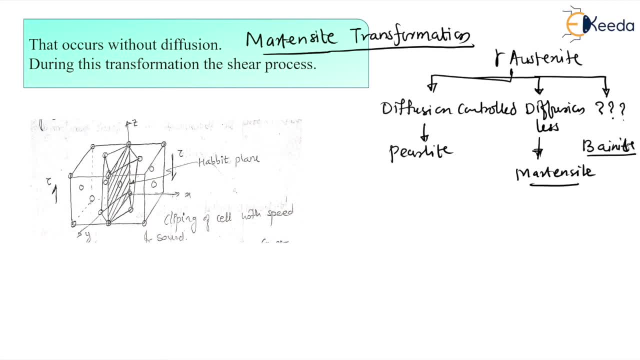 Because, no, any correct Explanation for this phenomena is still there, But even though many of the scientists or authors have given the literature for the same. that is the bainitic transformation. but, dear students, just now we have- in the previous videos we have talked about the austenitic diffusion- controlled transformations, that is, the pearlitic transformation. 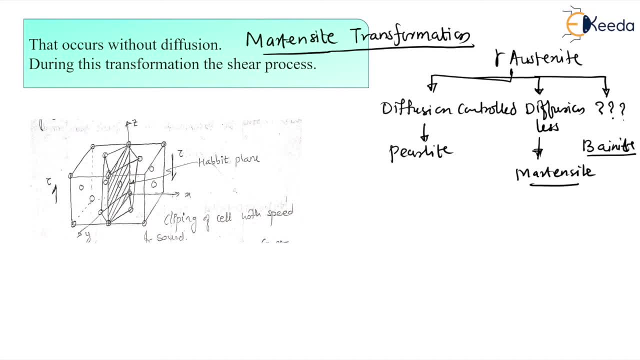 Now let us talk about this martensite transformation, dear students. So actually this transformation was given by the German scientist R Martens. who gave this R Martens? okay, Actually, while doing the experiments on the pearlitic transformation, only Martens investigated or invented this martensite phase. okay, dear students, 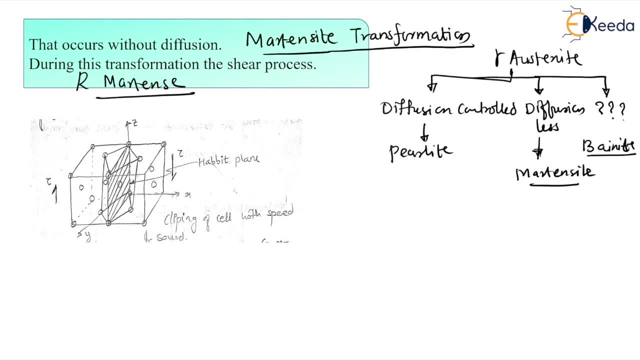 So, dear students, this martensite is actually the separation. So this martensite, dear students, is actually the separate phase. And as we know that the pearlitic transformation is because of the diffusion of carbon atoms at the interstitial sites of this iron, 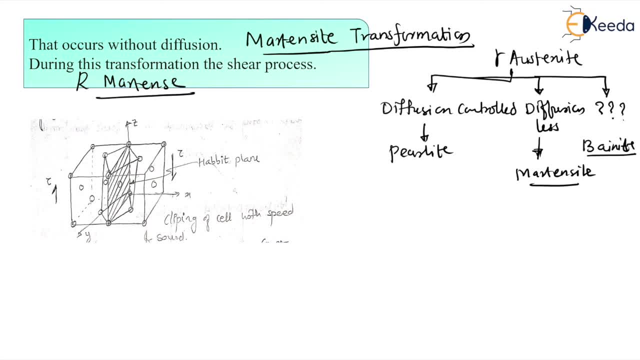 So definitely, dear students. we know that the diffusion of the carbon is definitely at very high temperature, But, yes, at the same time we have talked about this is not the infinite, okay, Because, if you know, diffusion is a time-dependent phenomena, it needs time, okay. so it's not like diffusion. 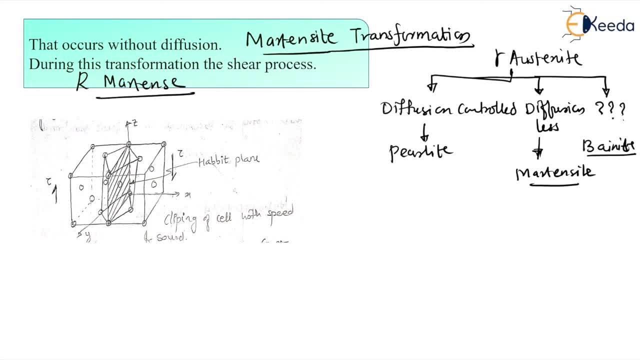 starts once, then it will continue for infinite period of time, because time always comes from high temperature to room temperature, isn't it so? for diffusion, we need time, and temperature is also very important. so now, dear students, what I'm saying, that our regular practice, what I'm saying, we are hitting this steel up to the same 950. 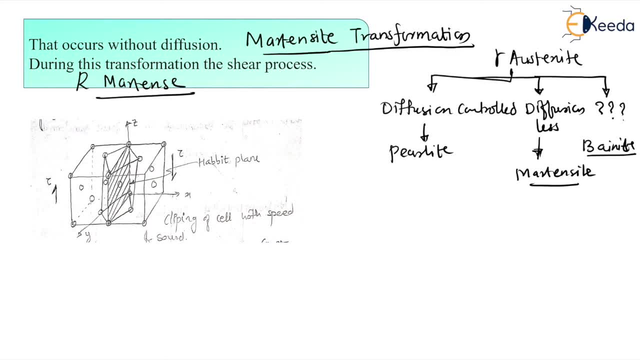 degrees centigrade. and here what we are going to do, that, that is, we are going to drop this temperature of the steel specimen from 950 degrees centigrade directly to directly, from 950 degree centigrade to directly, room temperature. okay, or Wobbeke, say, within the couple of seconds, within the couple of seconds. 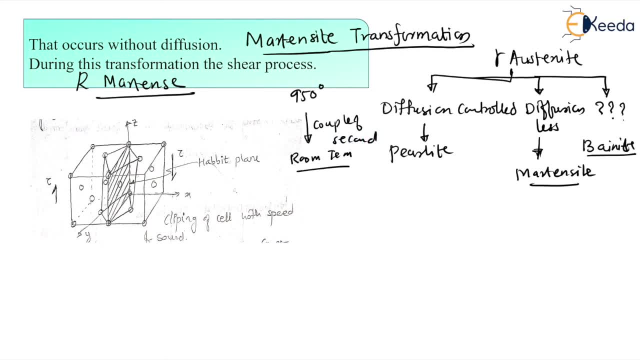 okay. or Wobbeke say within the couple of seconds, within the couple of seconds, okay. so, dear students, so till now, joby, I'm a discuss kiya uptick, so sorry, transformations way. yeah, gamma, I'm Nicky, I hope they were the guy. gamma, a one line. can each a cubby be stable? 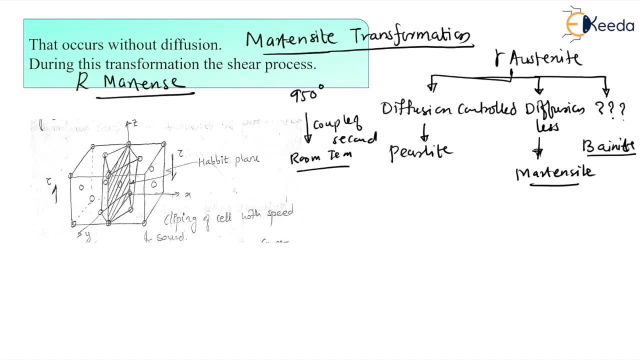 linear. so what? transfer, hojata, kiss me, cementite may, or dosa, tomorrow, alpha me. okay, that is the perlitic structure we are getting. but, dear students, yeah, happy may be the no time, of course, within no time may know so, but just degrees disintegrate. come here sample. 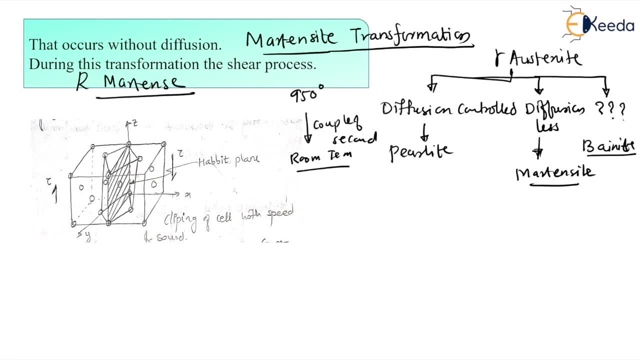 it may see those for character. now, quench Cara. of course I am quenching in the water bath, okay, and I am coming to the room temperature, so but our gamma, Kappa Jaigar, so definitely gamma copper stable area. so I will have one line gamma. 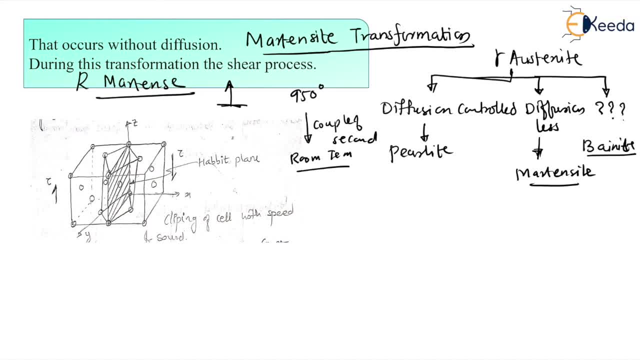 is stable there, okay, but make bad color me see the room temperature. be happy, Jahape gaama will be no more stable. so you have to go to a mix of getting the. So definitely it should be. get converted into something. Arre bhai, wo pata hai ki room temperature pe gamma kabhi bhi nahi bansakta? 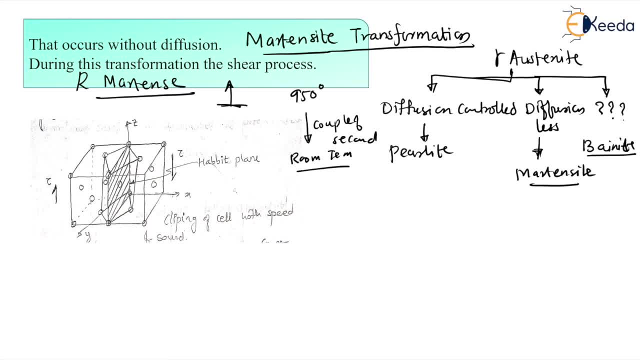 Gamma kabhi bhi stable nahi hai. That is gamma austenite ki baat kar raha ho May, yeah, austenite kabhi bhi room temperature pe stable nahi hai, Lekin phir bhi may bol raha ho ki may usko austenite ko at 950 degree centigrade se. 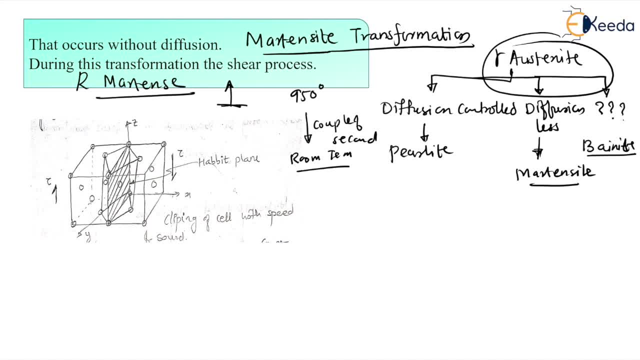 seetha within no time may usko room temperature me, la raha ho. So yes, this gamma has to be converted into something, dear students. So what I am saying? this gamma, this gamma has to get converted into something. 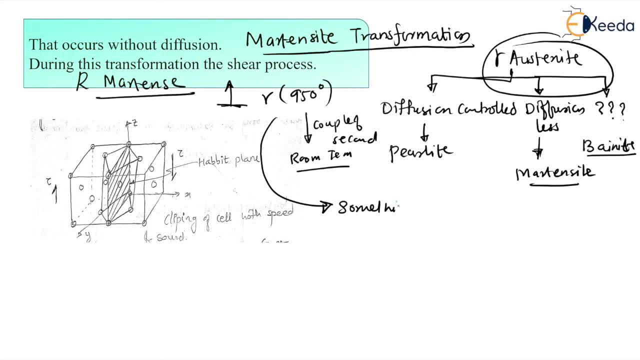 And, dear students, this something is nothing, but actually this something is known as the martensite. Yes, this something, dear students, is known as the martensite. Say this is the gamma which is having the face center pubic. 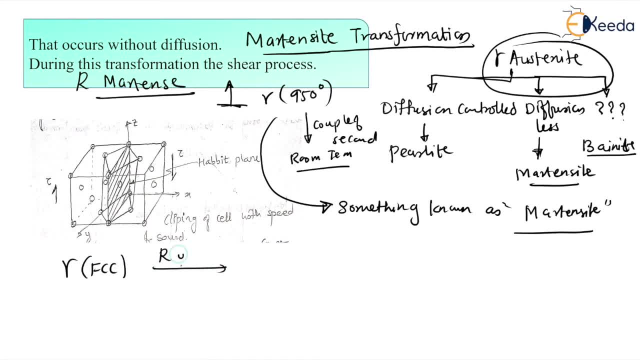 Structure. I am rapidly cooling it. I am having the rapid cooling of this gamma austenite to the martensite, As you know, that, as room temperature, only alpha is stable, isn't it? But here, this alpha is also not there. 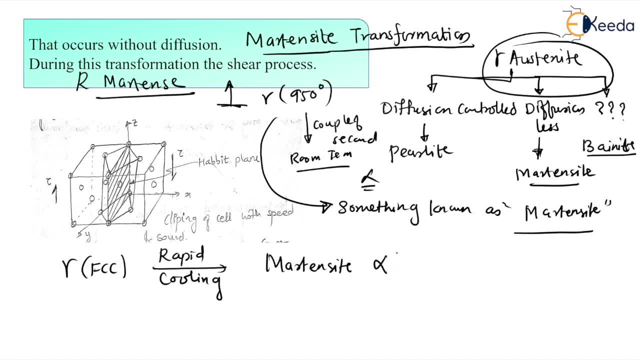 So it will be something like this alpha prime. I am saying, dear students, What I am saying: this will be the alpha prime which is having the body centered tetragonal structure. Kya hai ye? So how you read this alpha dash? that is nothing but the alpha prime which is having 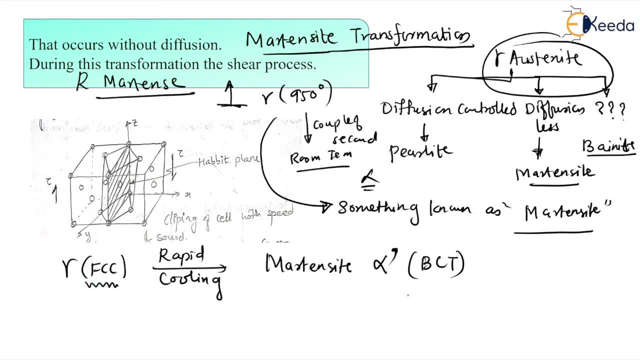 deko gamma austenite ka. kya structure FCC hai? seetha aapko kya mila at room temperature? jesa aapne usko cool kya? you got it as the body centered tetragonal. 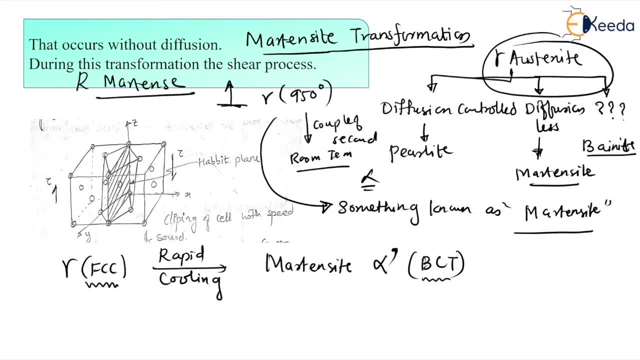 Ok, dear students. So, dear students, this transformation, actually it does diffusion, less transformation. Ok, aur usko aap ek naam bhi de shakto hai ki ye jo transformation hai, ye displacement or displacive in nature hai. 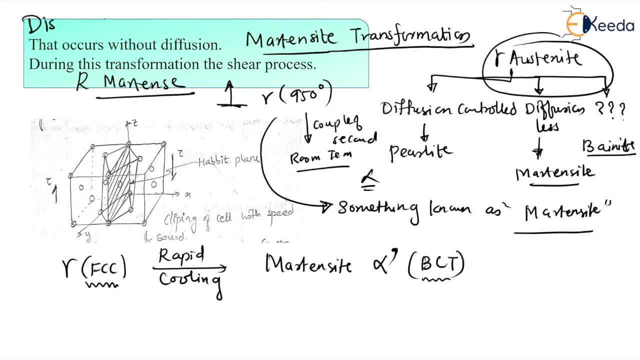 Kesa ye transformation Displacive in nature. Ok, so actually this happens due to the copper T property of the carbon atoms. Why it is happening? Because of the copper T property- We will see it how- Of the carbon. 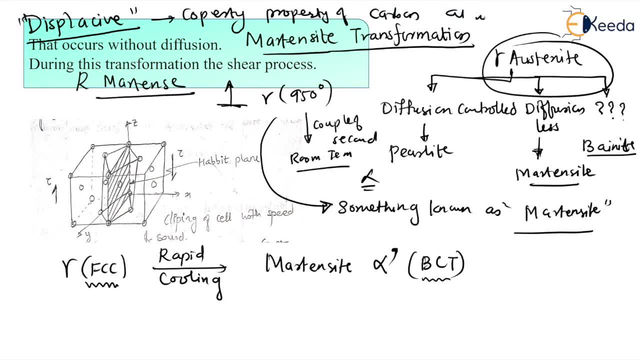 Of the carbon atoms, Of the carbon atoms. Ok So, dear students, so actually, this transformation occurs without any compositional changes. Ok, So, this transformation is a process of the shear that occurs without diffusion shear. So, dear students, during this transformation, this shear process is actually converting. 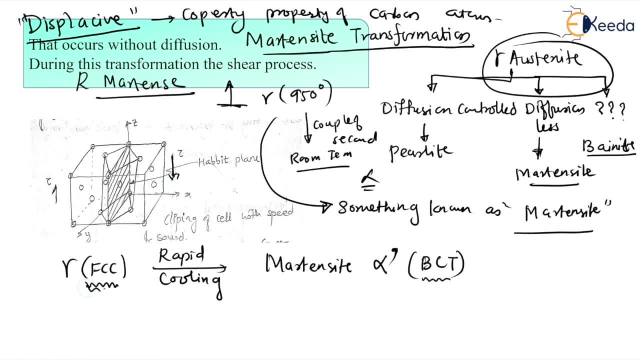 this FCC, This FCC Structure of austenite to the BCT structure of martensite. Ye kya hai iske piche mechanism, Ek to ye diffusion, less transformation hai To hai kya ye Ye displacive transformation hai. 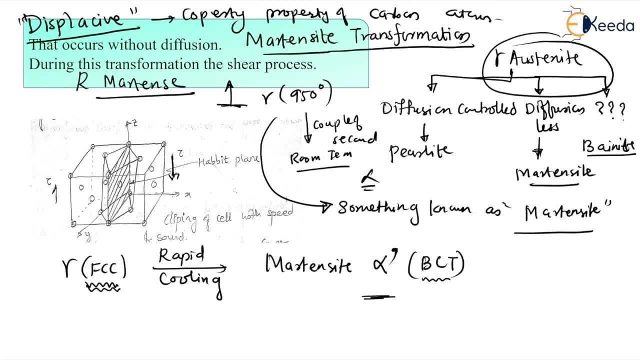 Aur ye kis ki wajah se ho raha hai. It is because of shearing. Ok, So let us have this the well suited diagram, dear students. So main hai kya, kya Ye haan pe. main hai do gamma austenite ke FCC. 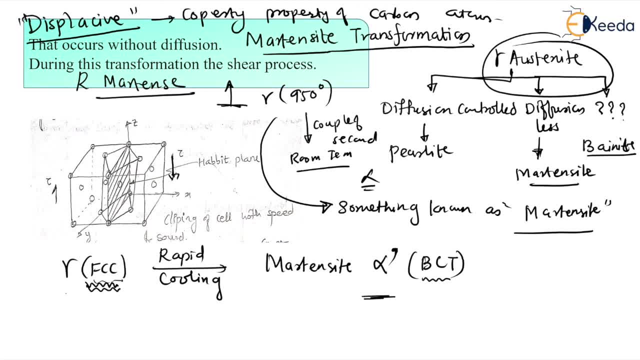 A sales way. Ok, So you can see, here I have taken this two FCC of this gamma austenite, gamma austenite. Ok, Like this. So ek ke bagal mein main, ek dekha aise bohut saare, this side hai, this side hai. 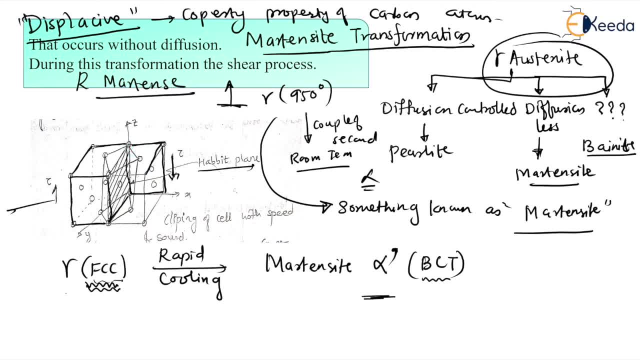 Ok, Ok, Just, we have taken two which are adjacent. They are adjacent to each other: FCC units, Unit sales Like this, Aur FCC mein kya hai Aat corner pe aat item to hai hi. In addition to that, we are having on six faces of cube. we are having har ek face pe ek. 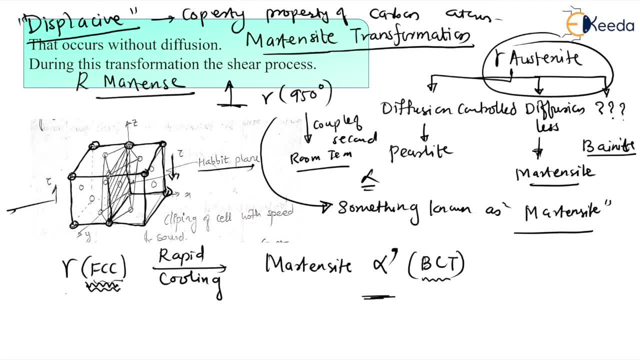 Barabar, That is a face centered cube. Now, dear students, So ye jo yahaan pe, when we are quenching this Sample, this austenite from 950 degree centigrade to this room temperature, So see here what is going to happen. 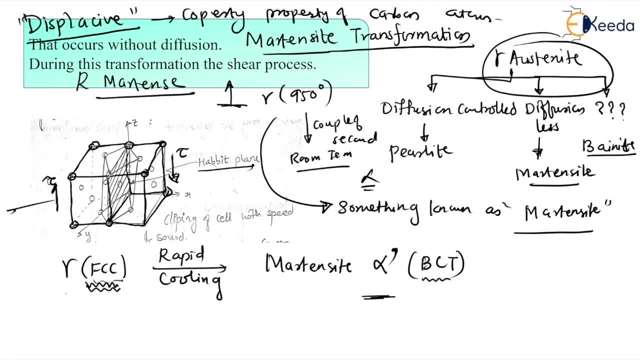 So same thing here, dear students. I am showing you the mechanism. actually, This is the shear, because this mechanism is going to happen with the shear. Ok, So see here, when we apply the shear, that is, we are quenching it. 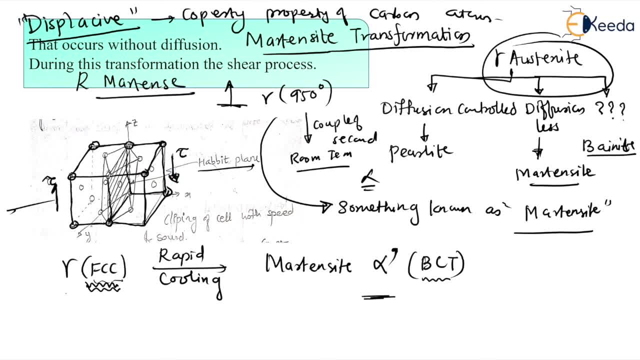 So what is going to have to happen here? So this, Say this: This is the x axis, This is the y axis And this is the z axis. Ok, So, dear students, this because of the shear stress this sales are going to have the clipping action. 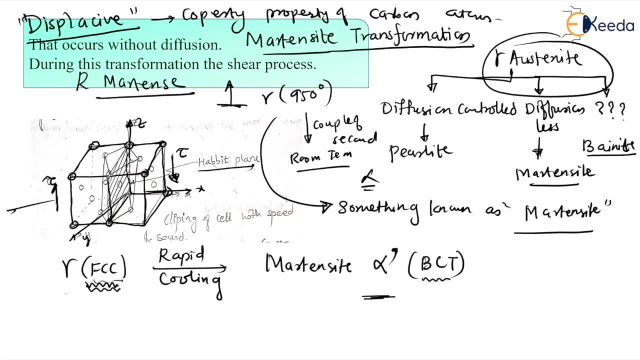 Ok, They are going to clip Like twisting a Twisting the fingers. Ok, Like twisting of this, all this FCC sales, Ok, So here, what is going to happen, dear students? These all the sales are going to clip with the velocity of sound when you quench it. 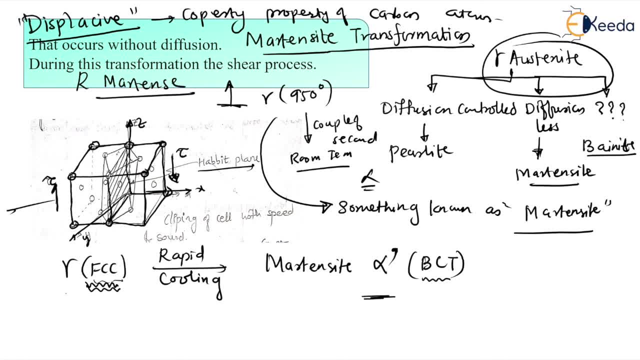 And see here what is going to happen. Here we are, we will be getting this. So only the required atoms on the face we have shown here to get this body. central tetragonal structure, when the sales are clipping like this. 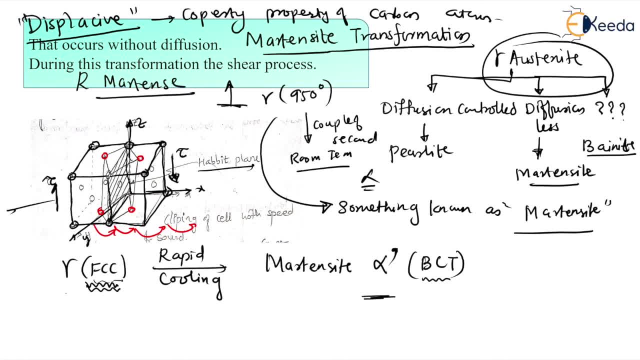 They will clip like this, with the period of sound. And here, students, if you see, here we will be getting this tetragonal. This tetragonal, We know, tetragonal means what A is equal to B, But not equal. 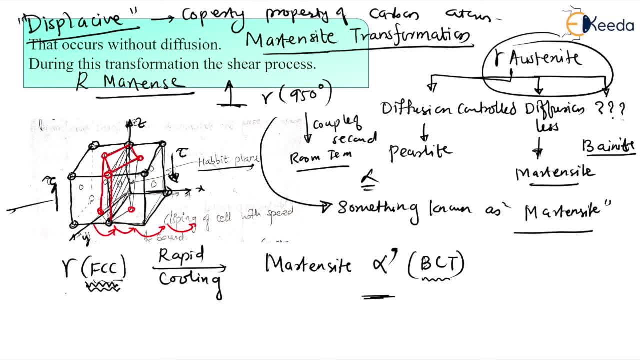 To C. So A and B are equal, but not equal to C. So you can see here, this is the body, central tetragonal structure, dear students. Ok, And dear students, so while doing or while having this clipping movement, so there will be the plane which will not change in any of the sales, dear students. 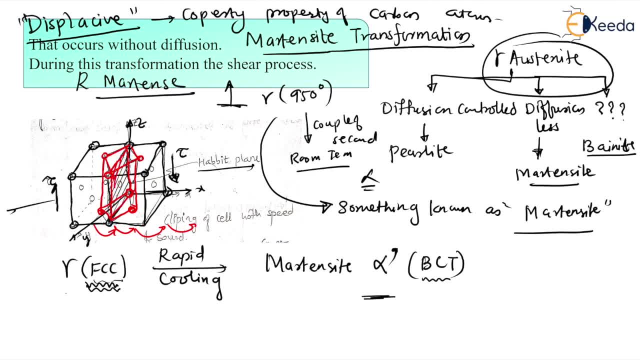 So, which is with the hashed light. So, dear students, that plane is known as The habit plane. Ok, So, that plane is known as the habit plane. So you can see, dear students, during this transformation, actually, this Z axis is subjected to 20% compressive strain. 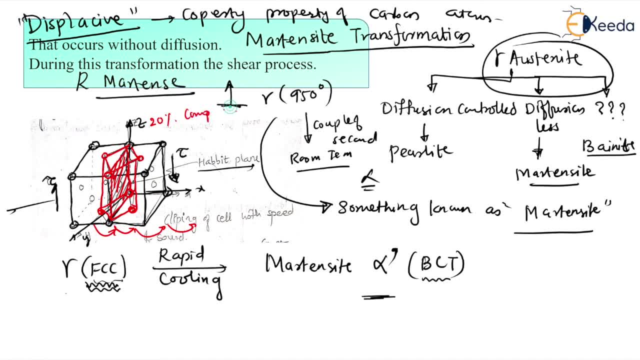 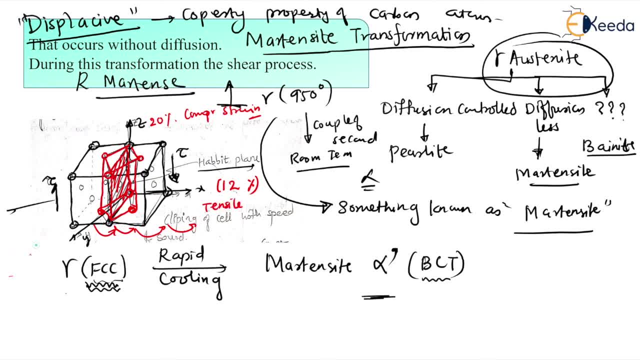 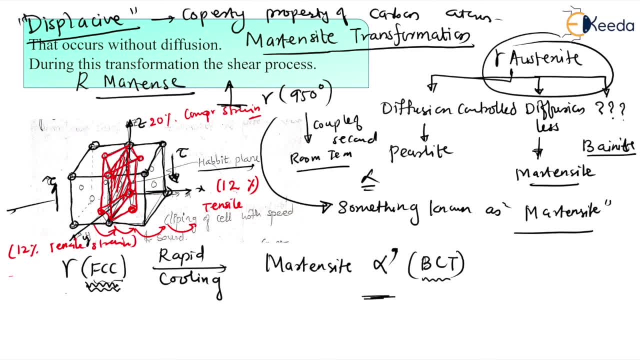 So, dear students, this is the homogeneous plane transformation. Ok, So here one plane will. So, dear students, so here, this one plane will remain undistorted, Before and after the transformation we have already shown here. 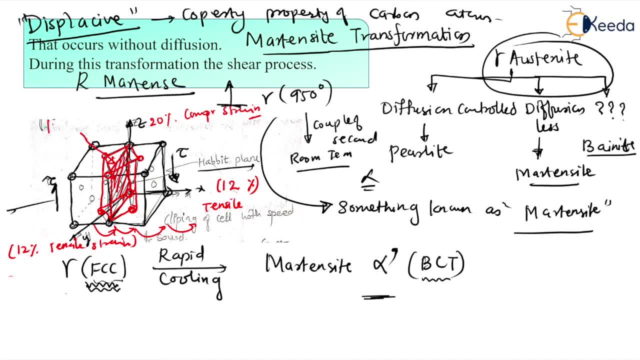 So, before and after the transformation, this habit plane is not going to get distort Habit plane, So it will not going to distort. This is the habit plane we already discussed, dear students. Now, dear students, if we look at the tetragonality of this BCTC plane, we can see that this is 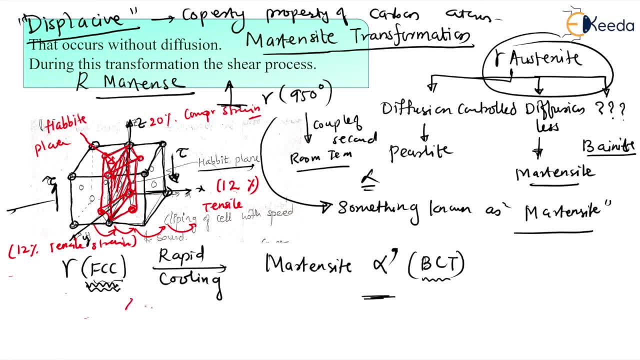 a tetragonal structure which will be dependent upon the percentage of carbon. because this is a tetragonal structure, That is, A is equal to B, not equal to see an angle R, alpha, beta and mR 90 degrees. 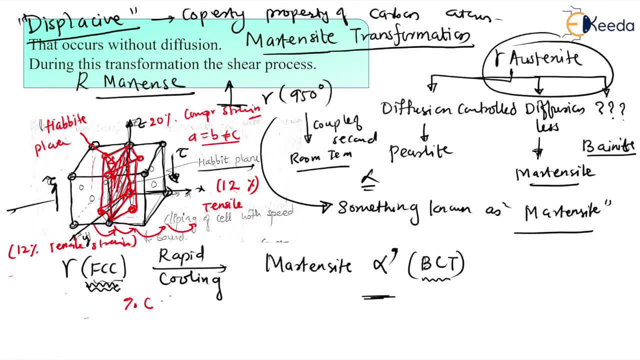 Ok, So, dear students, so here this tetragonality of this BCT structure, body, central tetragonal structure is basically dependent upon the percentage of carbon in the steel, in the steel. Ok, Ok, So we know the tetragonality. 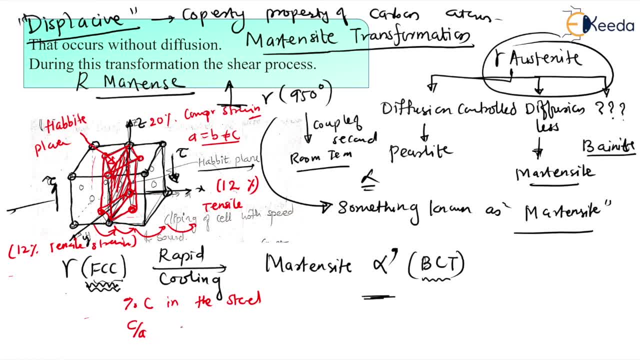 So we know the tetragonality by the ratio C, by A ratio which is equal to 1 plus 0.045, into weight percentage of carbon. weight percentage of carbon. So, based on this formula, dear students, this tetragonality is actually dependent. 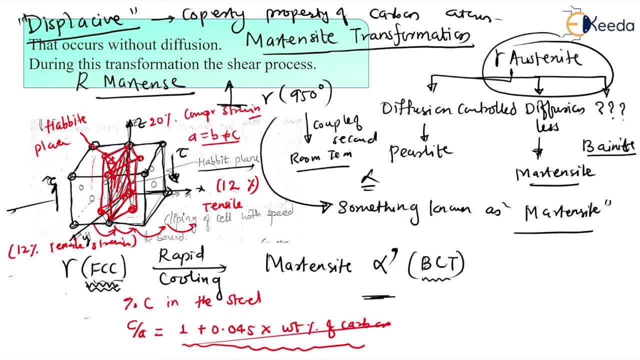 Ok. So, dear students, suppose, if I take the example that say I am having 1 percentage of carbon, I am having 1 percentage of carbon. So tell me what will be this tetragonality, That is, C by A ratio, will be what for 1 percent? 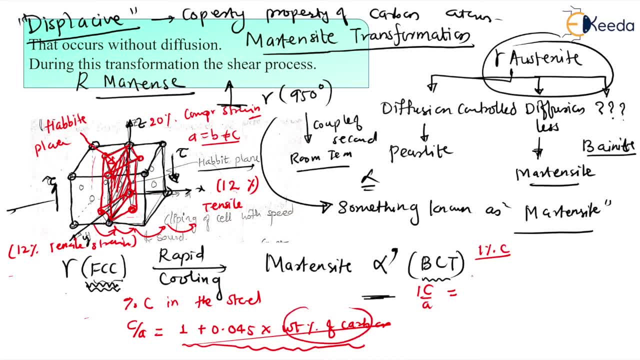 So put here weight percentage of carbon as 1,, you will get 1.045,, isn't it So, dear students? by this C, by A ratio, this martensitic transformation for very low carbon steel, ok, what will be there? 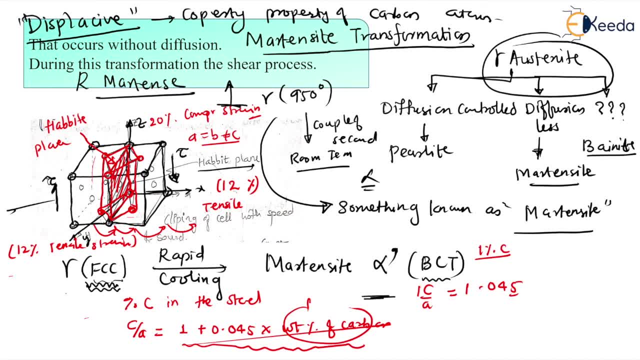 Very low carbon steel. if I go, dear students, this bhale martensitic transformation, mein humko martensite ka structure mila BCT, But jaha pe C by A ratio nearly equal to 1 hai waha pe kya milega apne ko wahi martensitic. 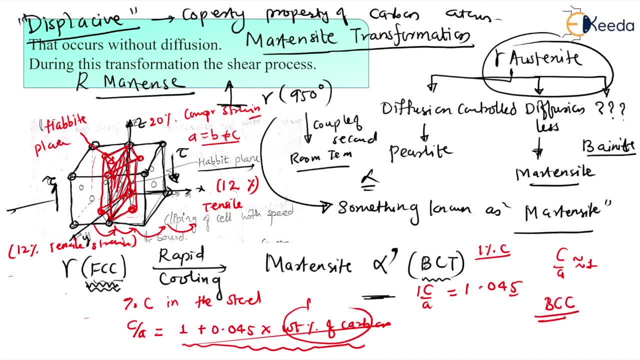 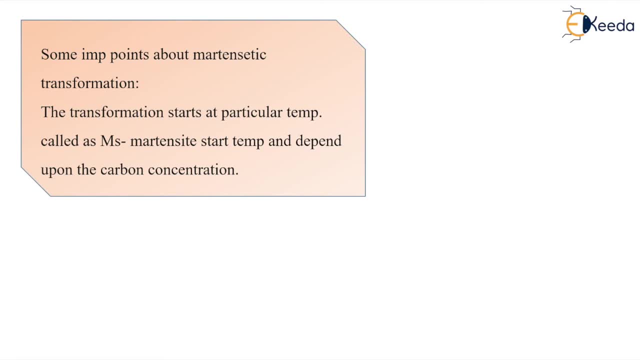 structure in the form of body centered to BCT. So BCT will be no more there, So there will be the body centered tetragonality, isn't it? So that is the thing, dear students, So, dear students. now, this is the way actually this martensitic transformation is happening. 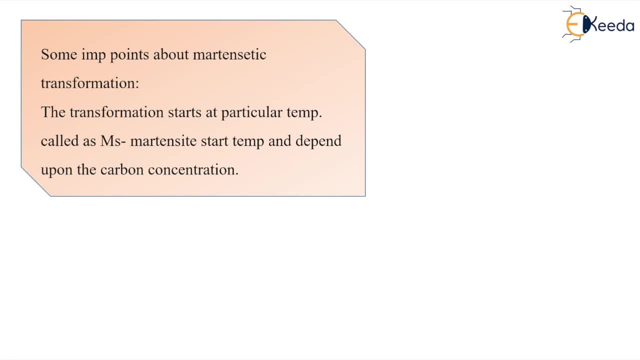 So here, no, any diffusion of carbon at the interstitial sides of the iron. Here only the thing is that the cells of the face centered, cubic cells of gamma austenite, they are going to displace, they are going to distort when they are getting quenched. 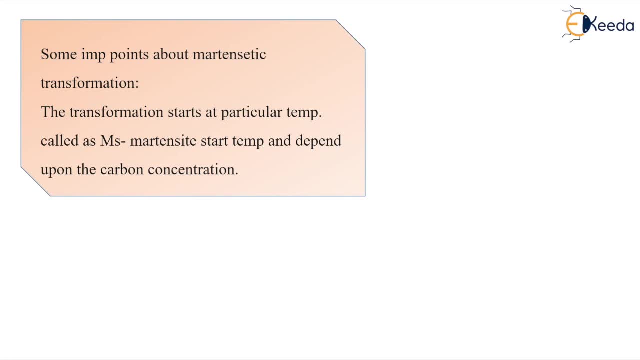 ok, And there will be what? The clipping of the cells with the speed of sound, and that will convert this FCC structure into body centered tetragonality, Or jitna carbon content. kam hoga steel mein utni hi yo BCT jo hai wo martensite ka jo structure. 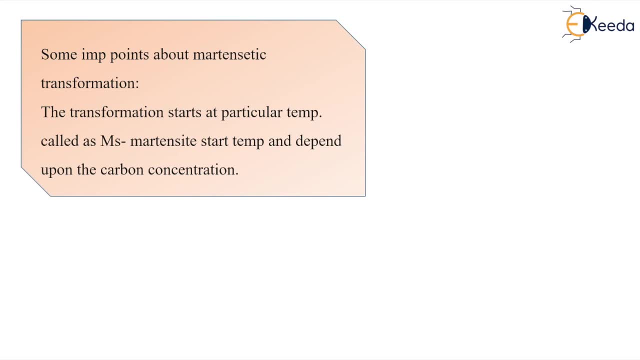 hai wo kya banta chala jayega body centered QB banta chala jayega. ok. Now, dear students, let us discuss some very important points about the martensitic transformation. ok, So the first point, dear students, that we have see, this transformation starts at particular 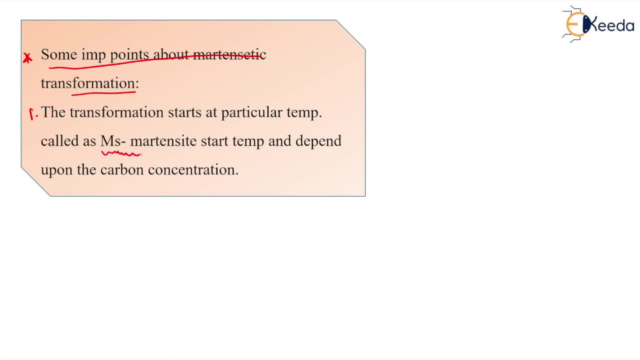 temperature, And that temperature is known as MS. that is martensitic start temperature. And again, it is going to finish at at particular temperature, and that point or temperature is known as martensite finish temperature. ok, So here jo, martensitic start temperature. hai, it will depend upon the carbon concentration. 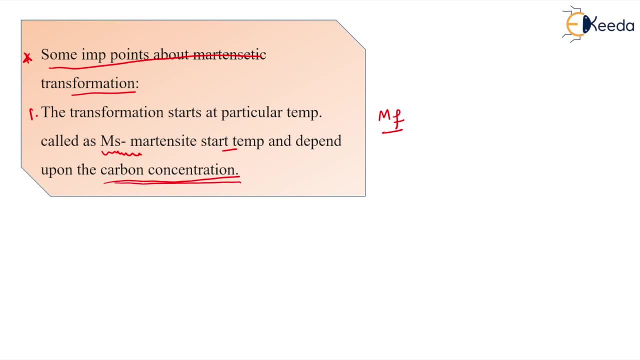 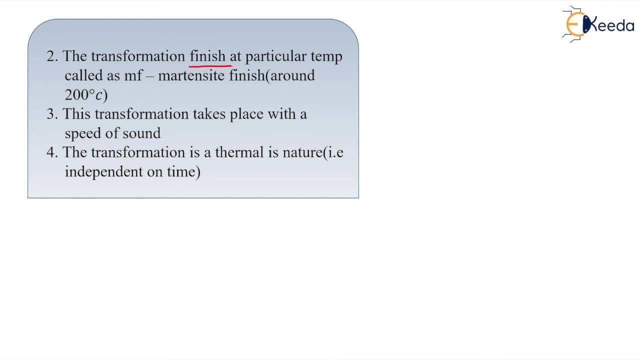 On the basis of this carbon concentration, we will get that temperature. In same fashion, dear students, this transformation is also having some particular finish temperature. that is known as the MF martensite finish, which will be around 200 degree centigrade. 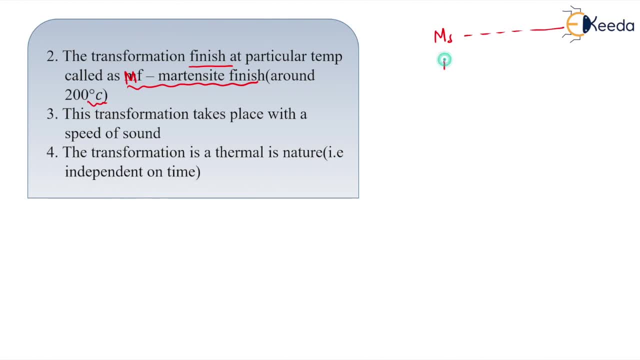 So martensite start will be temperature will be there and martensite finish temperature will be there. This will be around 200 degree centigrade. ok, So, as I told you, this transformation takes place with the speed of sound that is clipping.